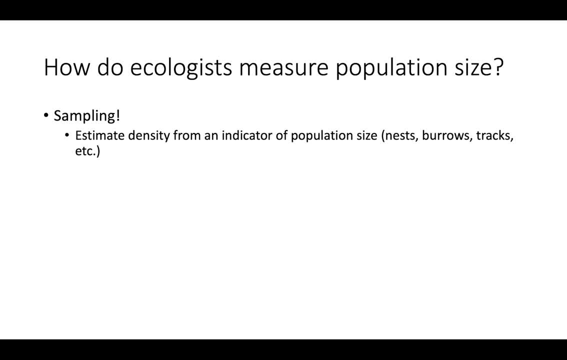 of indicator of population size, such as the number of nests, the number of burrows, tracks, animal droppings and things of that nature. And then the second would be mark and recapture. So in mark and recapture, what they do is they'll catch organisms that they're concerned. 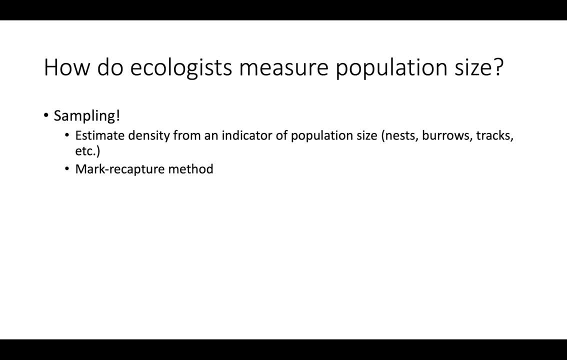 with and mark them somehow and then release them back into the environment and wait however long they want to- a couple days, a couple weeks- and then they'll go out and try to catch organisms again, And then based on the proportion of marked individuals in that second. 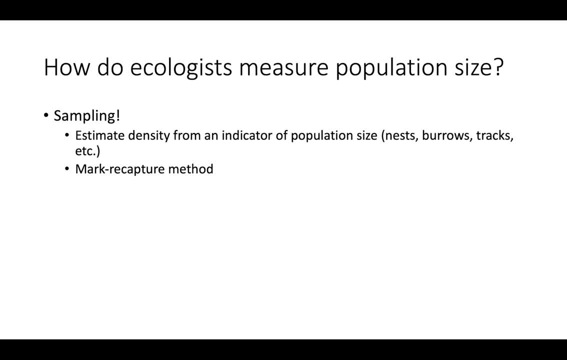 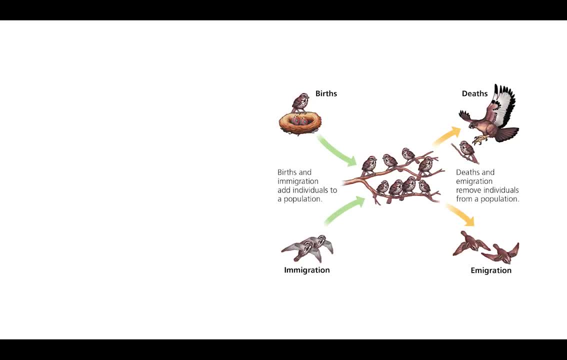 capture, they can extrapolate what the overall size would be. And so why do ecologists even want to measure population size? So the reason they want to measure it is because population sizes, population density, are constantly changing as individuals enter and leave these different populations And so over in this diagram. it's kind of 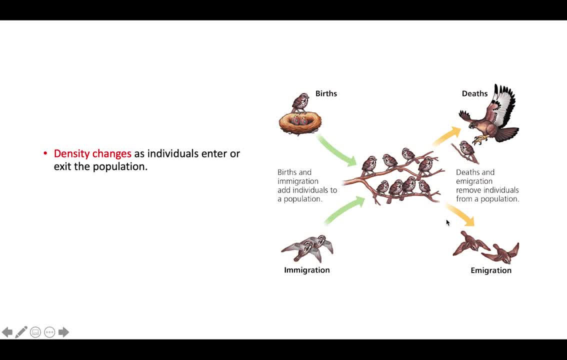 a visual depiction of how populations grow and then shrink, And so additions to a population are going to come from births and immigration. So immigration is going to be just individuals coming from a different area and moving into this population, And then removal of members from a population is going to occur through. 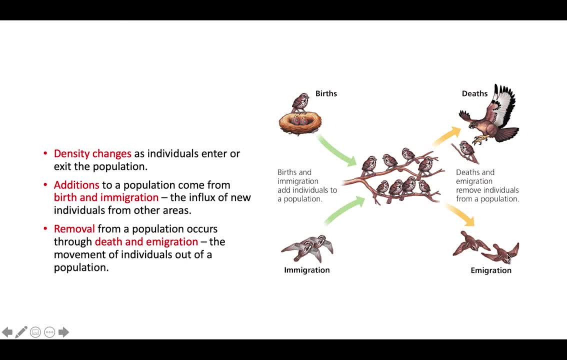 death and immigration, And so sometimes people get these two terms confused just because they sound almost identical, And so I was always told that to remember that this immigration means to leave a population is that it starts with an E, And so you can think of it as leaving a population, And so you can think of it as leaving a population. 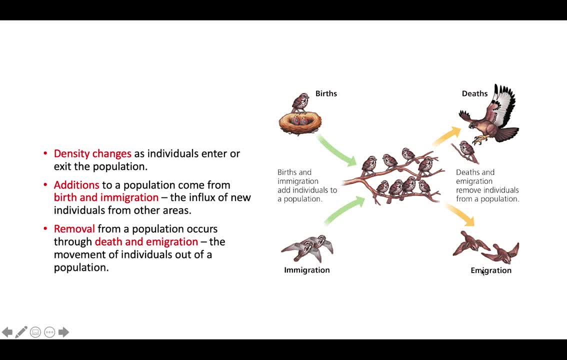 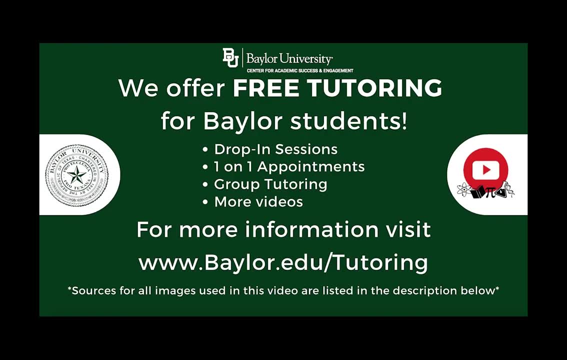 Think E for exit. So those individuals are exiting that population and then going to a new area. I hope you found this video really helpful. The concepts and information presented in this video will be true no matter what biology class you are taking. However, the concepts 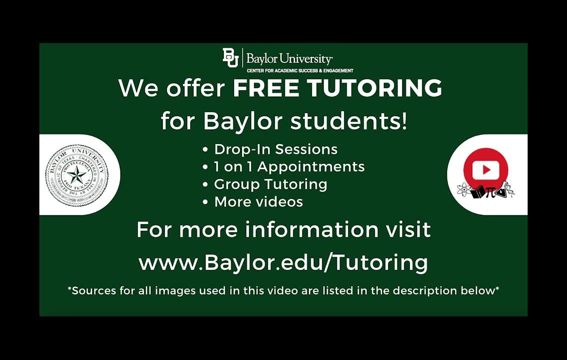 presented in this video are referencing material currently covered in Baylor University's coursework. Remember, if you are a currently enrolled Baylor student, we offer free tutoring services in our tutoring center, which is located on the first floor of the Sid Richardson building. You will find all the details you need about these services on our website, which is wwwbayloredu.